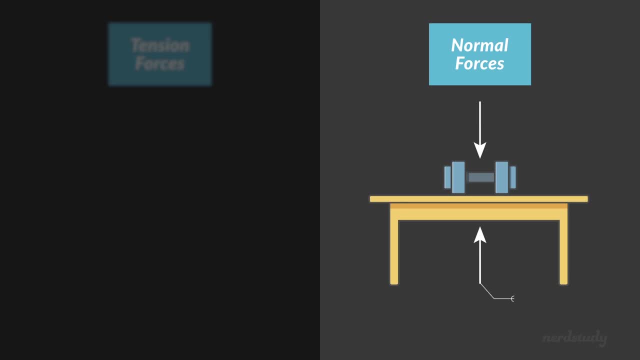 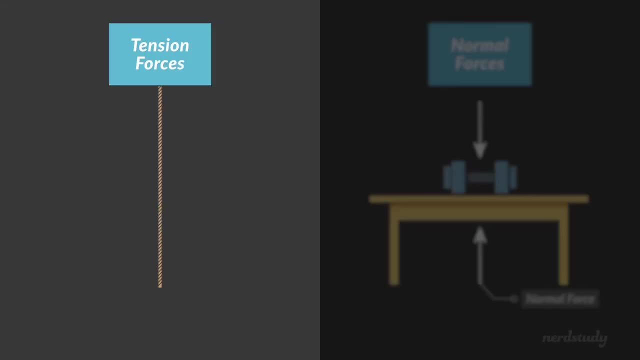 prevents an object from moving into the surface, and we call that the normal force. Tension forces do something quite similar, except that, instead of resisting compression, they resist forces that cause things to stretch. For example, when we hang a ball on a rope, the rope applies a force to the ball, which 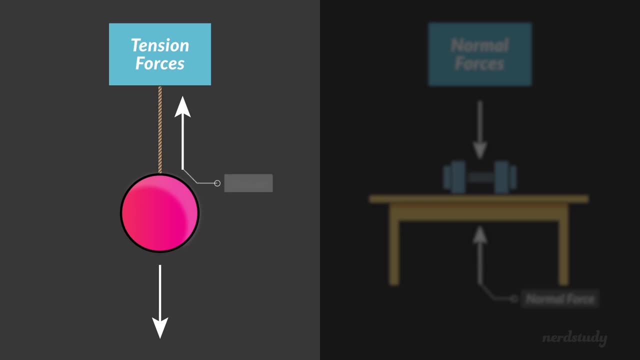 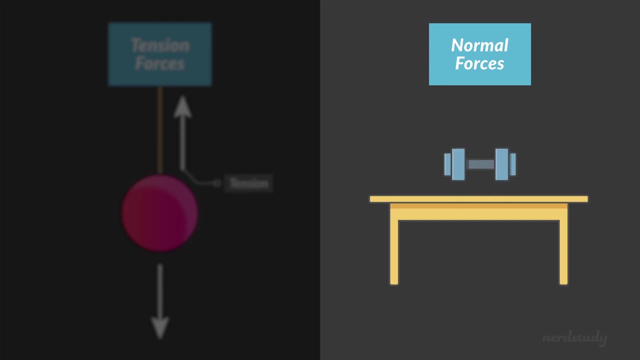 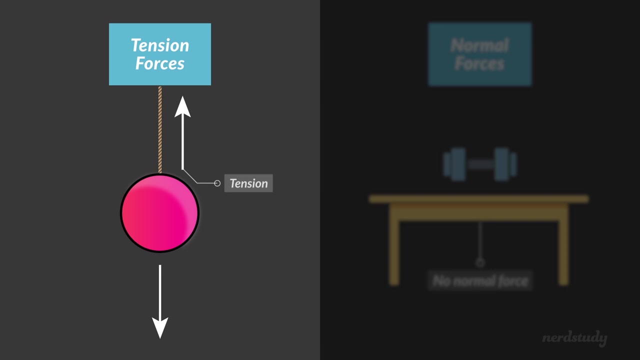 makes it resist being stretched out. The result is tension. Looking back at normal forces, it seems obvious that when an object is not pushing against a surface, the normal force must be zero. Tension forces are similar to this, but in an opposite sense. 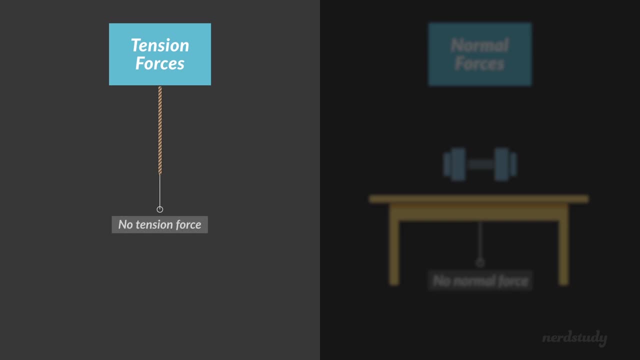 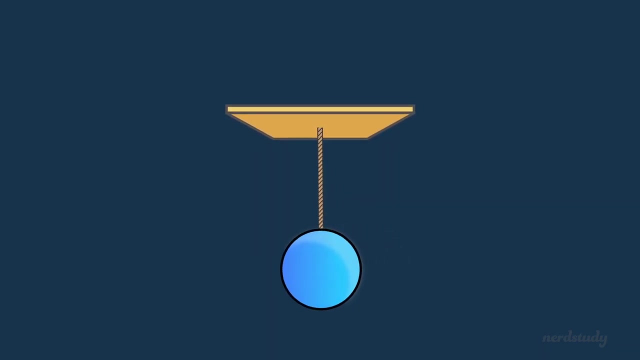 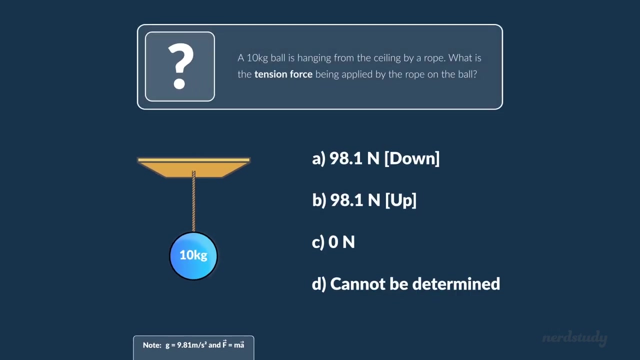 If an object is not pulling on a rope, the tension force is zero. Alright, I think we've got enough knowledge to look at a very simple example. Let's look at the ball on a rope again. If the ball has a mass of 10 kilograms, what is the tension force? 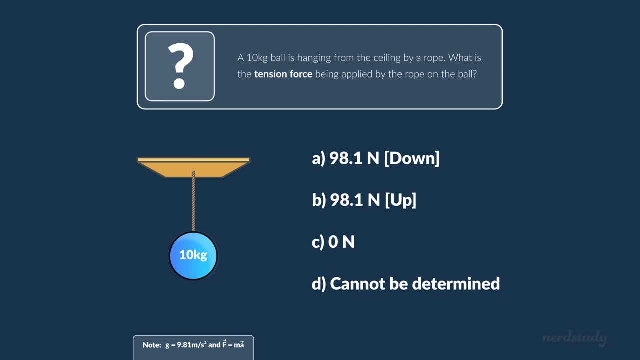 Hmm, how would we solve a question like that? Well, the answer would be 98.1 Newtons upward. How did we get that answer? First of all, we have to know the tension force. We have to look at the forces that are acting on the ball. 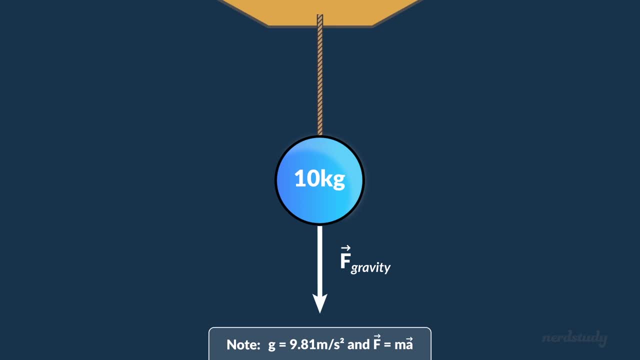 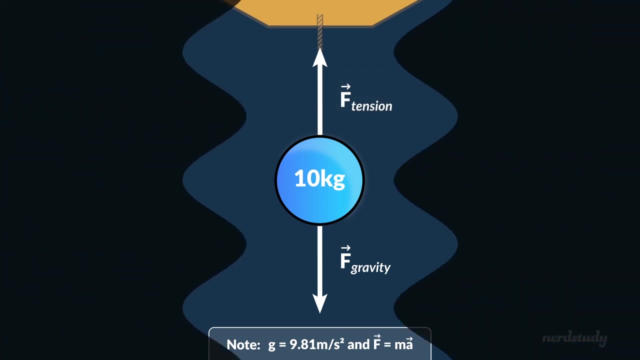 One of them is obviously gravity. What other forces are there? Well, there's really only one other force: The force of tension. More specifically, it's the tension force being applied by the rope onto the ball, And since the ball isn't moving, the forces must cancel out. 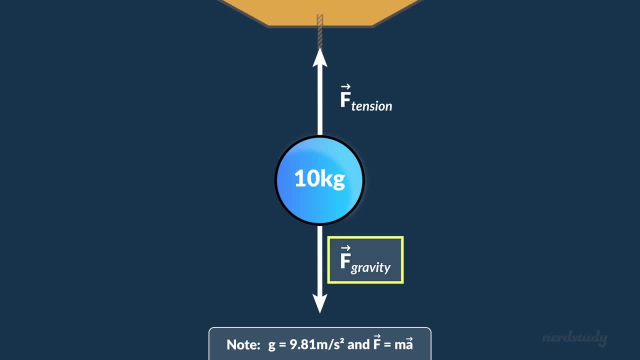 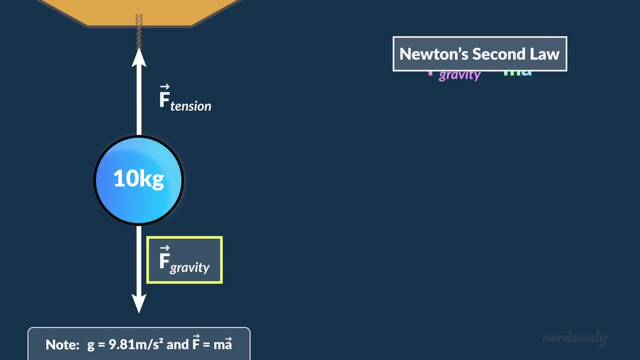 So our next step will be to find the force of gravity on the ball. Cool. To find the force of gravity, in other words the weight, we'll need to use Newton's second law. We already know the mass of the ball, which is 10 kilograms. 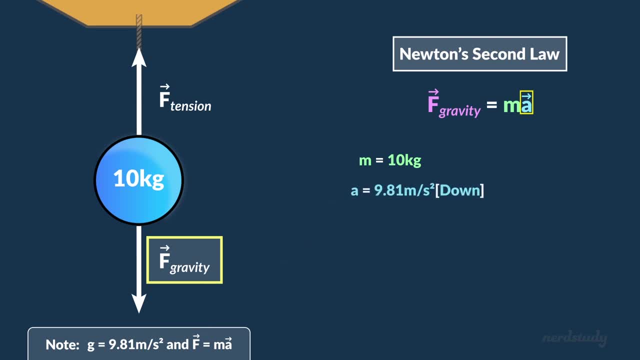 As for the acceleration, that's constant near the Earth's surface, which is 9.81 meters per second squared downward, And once we substitute those values into the equation, we'd get 98.1 Newtons downward for the weight of the ball.